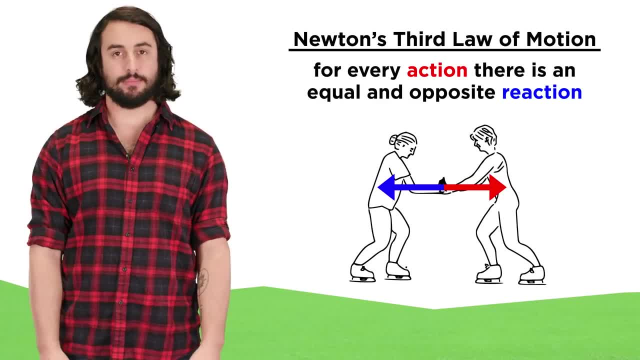 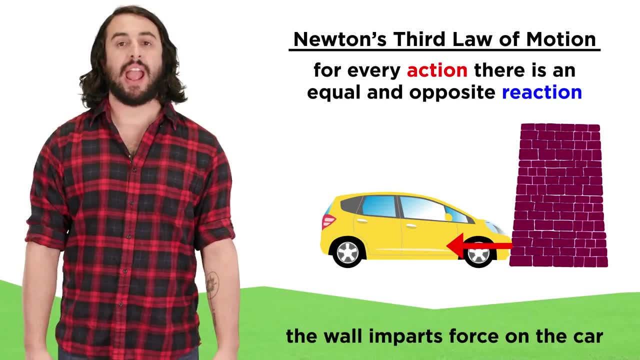 in magnitude and opposite in direction. Think of a car hitting a brick wall. The car imparts an action force on the wall from its motion. Then the wall imparts a reaction force right back on the car, bringing it to a quick stop. 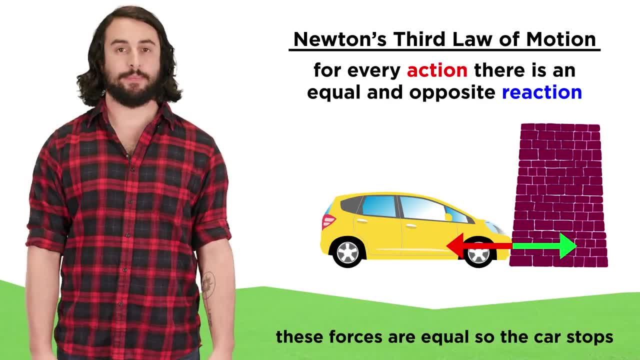 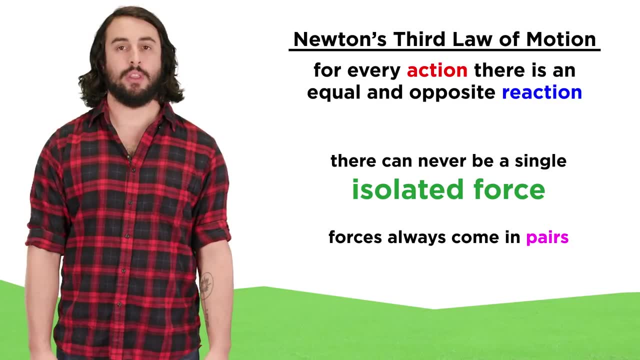 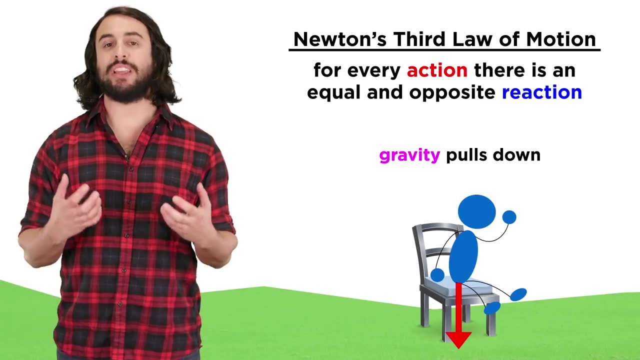 These vectors are equal in length and point in opposite directions. What this also means is that there can never be a single isolated force. as any force is an interaction, Forces must always exist in pairs. As you sit in your chair right now, the force of gravity is pulling you down towards the 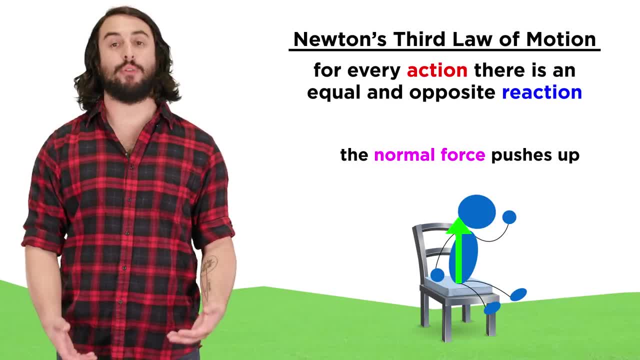 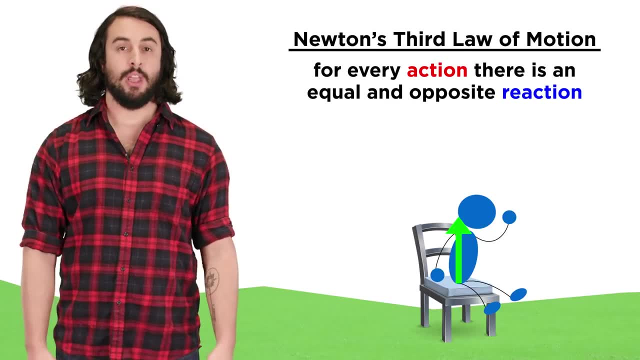 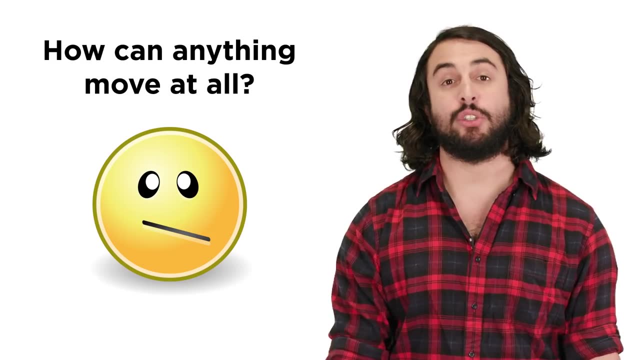 center of the earth, But something called the normal force points straight up with the same magnitude, which is why you remain perfectly still. We will learn more about this force later. The third law can sometimes be confusing, because it would seem to imply that no object. 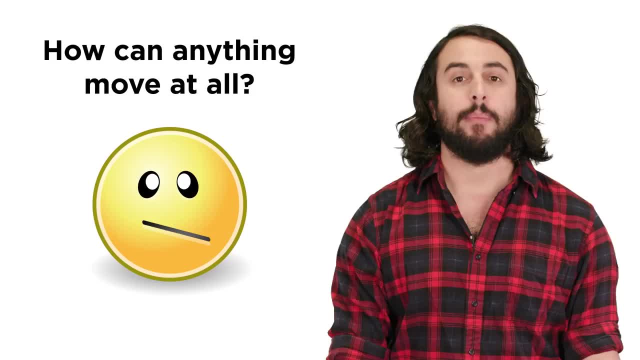 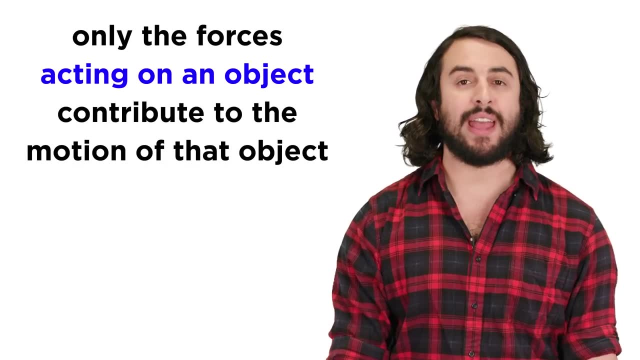 could ever move, since any force accelerating an object must be paired with another in the opposite direction. For this reason we must understand that when assessing the motion of an object, we consider only the forces in the motion of the object, We consider only the forces acting upon that object and not the forces that it applies. 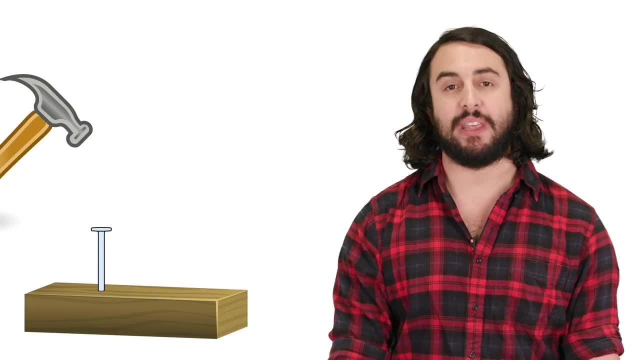 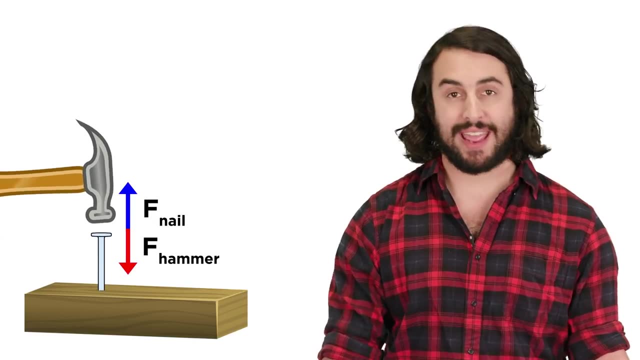 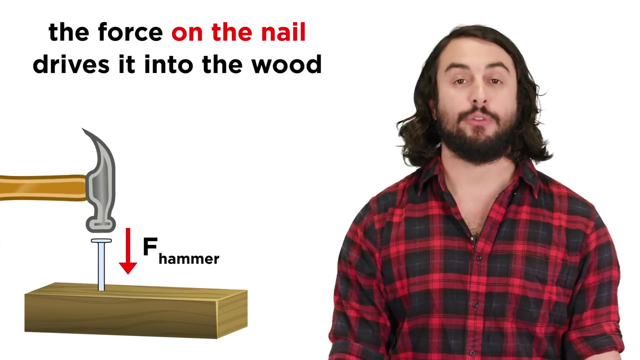 on other objects. When hammering a nail into a piece of wood, the hammer imparts force onto the nail and the nail imparts force onto the hammer, But the nail is driven into the wood because there is a net force acting upon the nail. 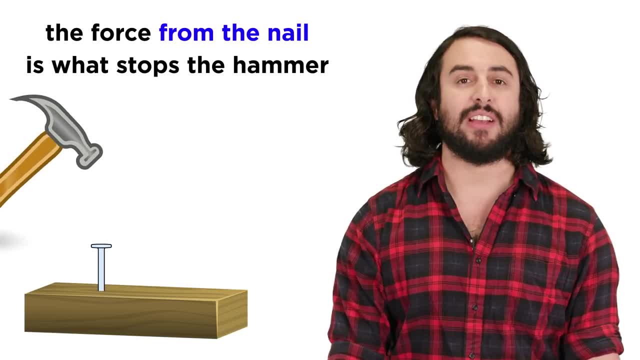 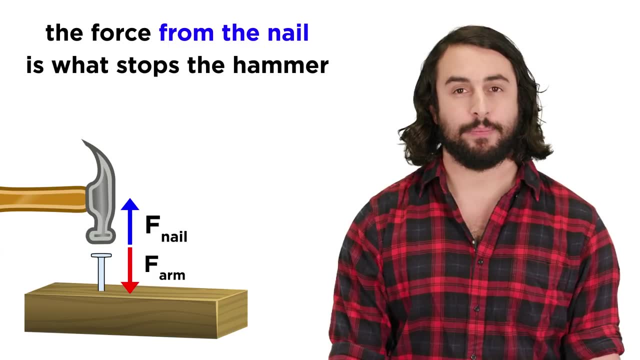 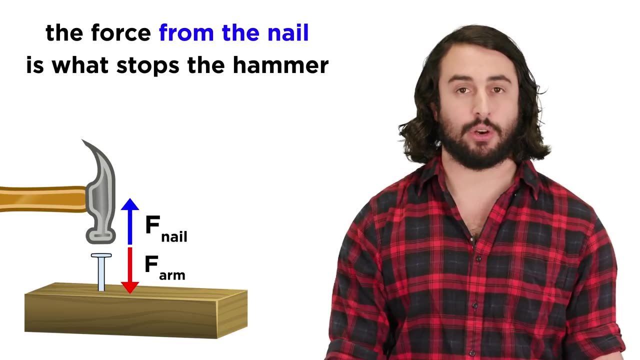 from the motion of the hammer. Likewise, the hammer has two forces operating upon it: The downward force from your arm and the downward force from your leg. That's why, when you strike the nail, the hammer stops moving at roughly the location where the impact occurs. 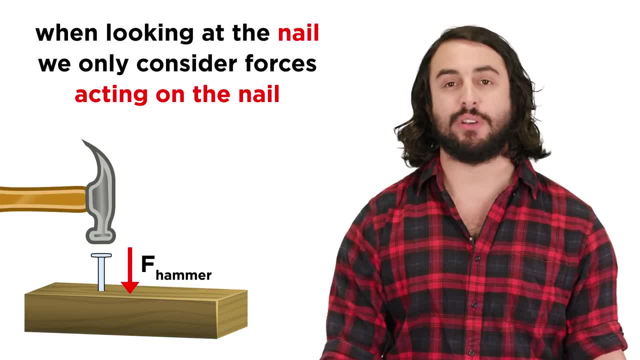 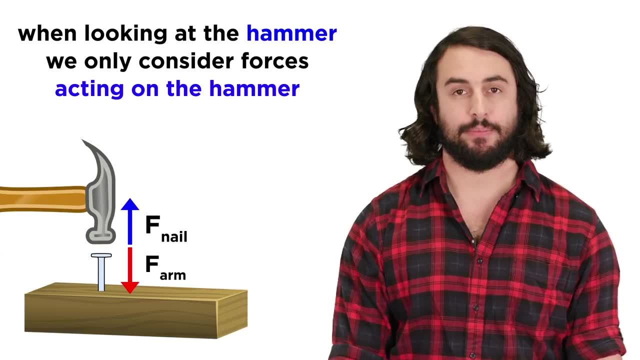 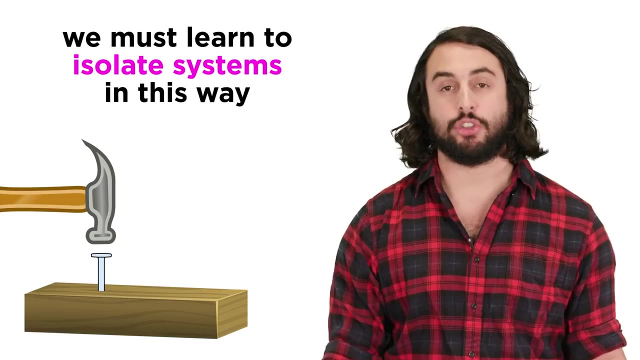 So if we are looking at the nail, we only consider the forces acting on the nail. If, looking at the hammer, we only consider the forces acting on the hammer. These are different systems, and this is the context in which the third law is best understood. 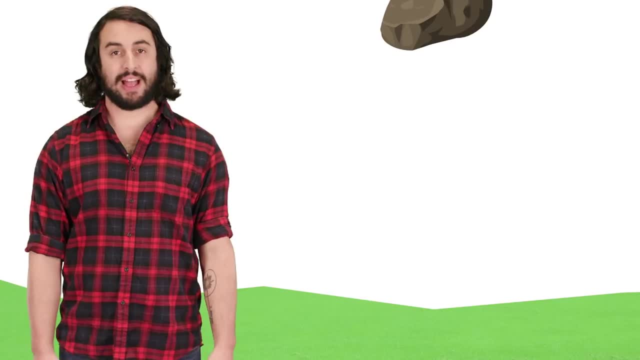 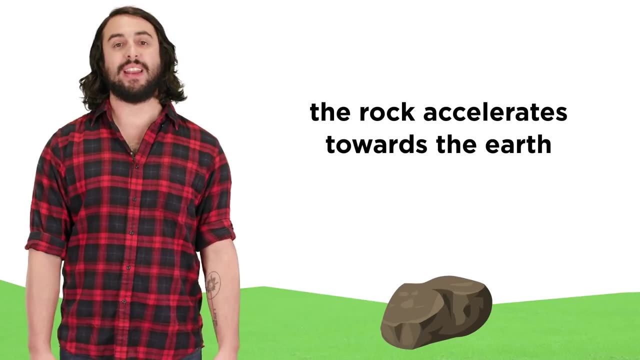 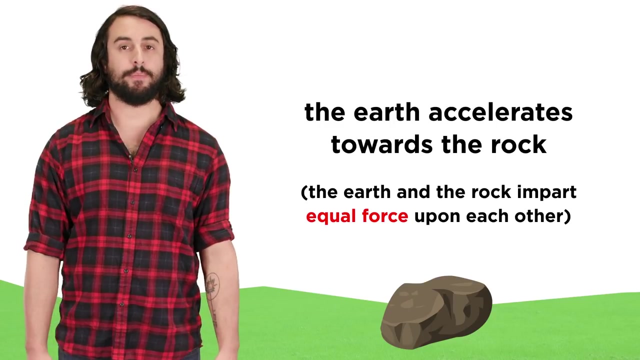 Let's look at another example. When a rock falls to the ground, the gravitational force from the earth causes the object to accelerate towards the earth, but it is also the case that the earth is accelerating towards the rock. This must be true, according to the third law.